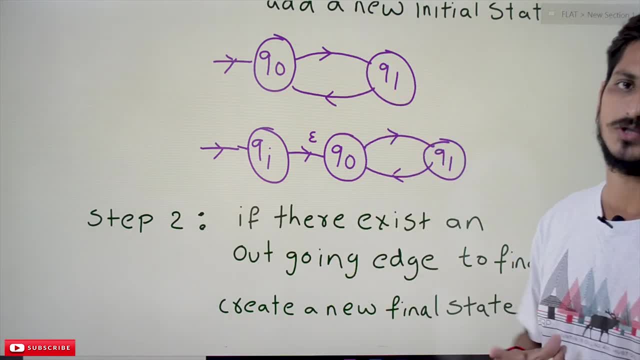 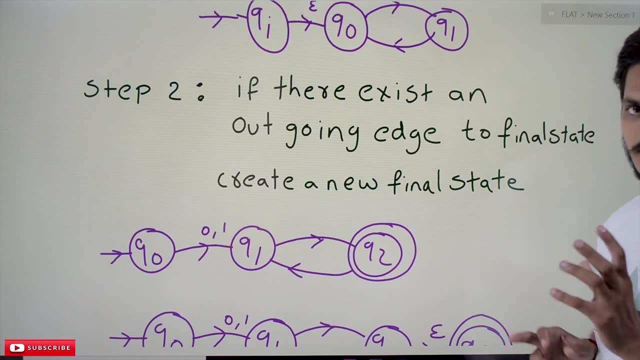 hoping that you already know what this DFA and epsilon moves- is Coming to the next step. if there is any incoming edge to the initial state, we are adding a new initial state. There exists an outgoing edge to final state. If there is a final state and if you are having 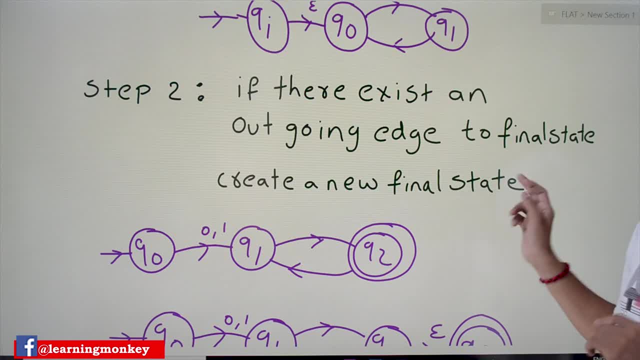 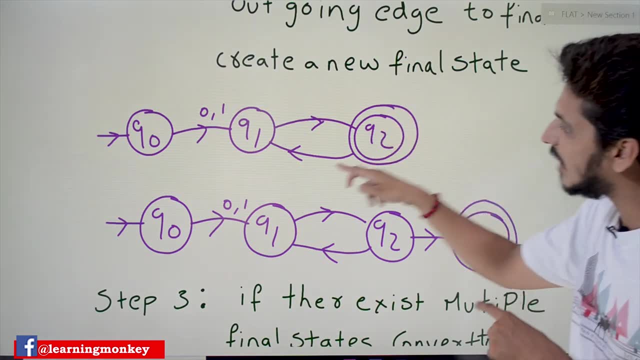 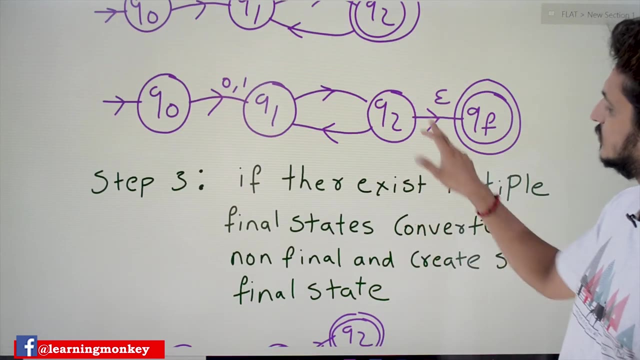 an outgoing edge to the final state, create a new final state. How to do that? Let's take an example: Q0, Q1, this is our final state. Q2 is having outgoing edge. So whenever you are having outgoing edge, create a new final state. So Q2 is taken as non-final state. 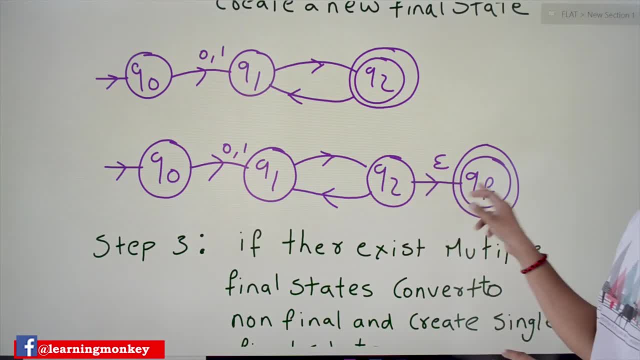 With this non-final state using epsilon moves, we are moving to QF. We created a new final state, QF, So now our new final state is QF. This is how we have to convert. Both of them are following the same logic. We are not changing the logic. 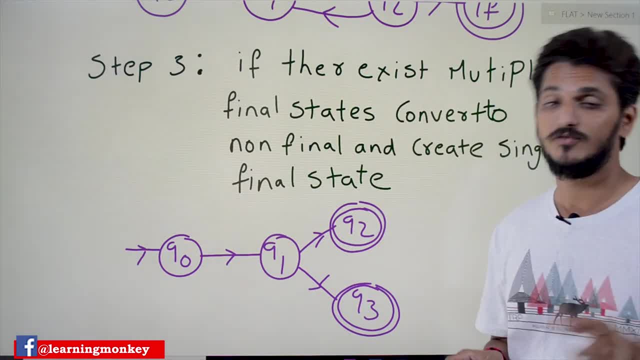 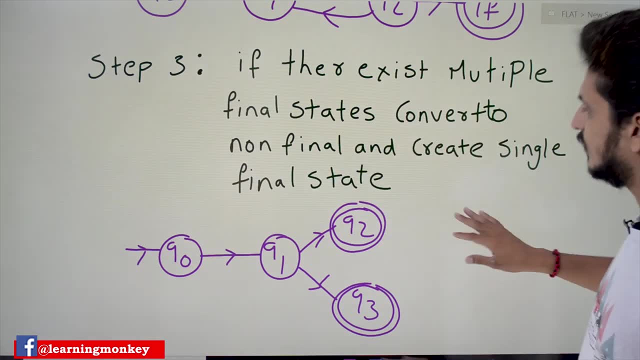 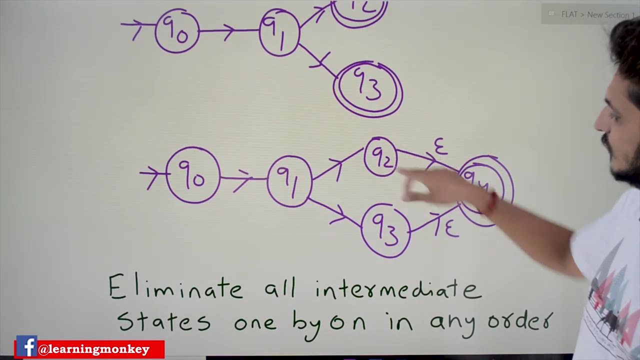 The next step is if there exist multiple final states. If you are having multiple final states, convert to non-final states and create single final state. Anyhow you will understand with an example. So if you are having two final states, multiple final states, we make it as a non-final state. 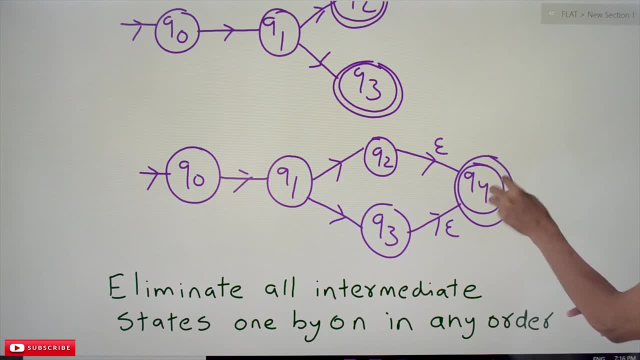 Using epsilon moves. we take a new final state and we make it as a new final state, single final state, using epsilon moves. So both of them are doing the same logic. This is the steps you have to follow, The three steps. after that, eliminate the intermediate states. 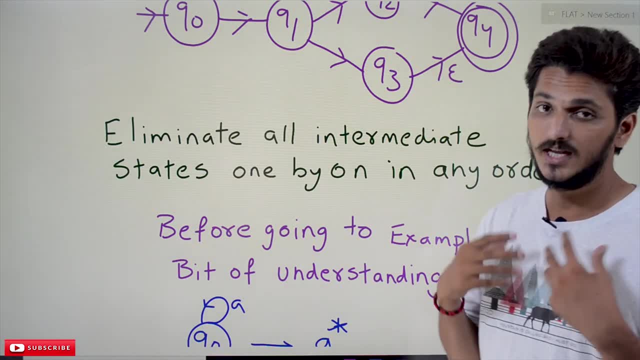 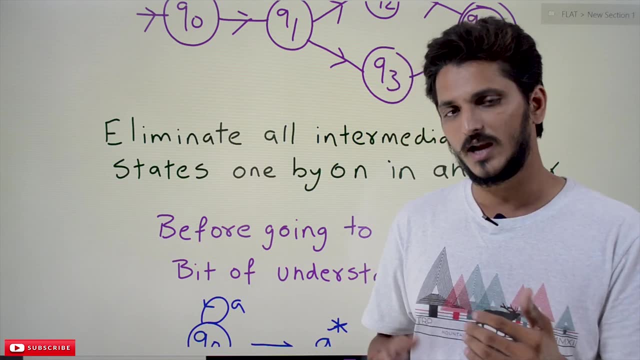 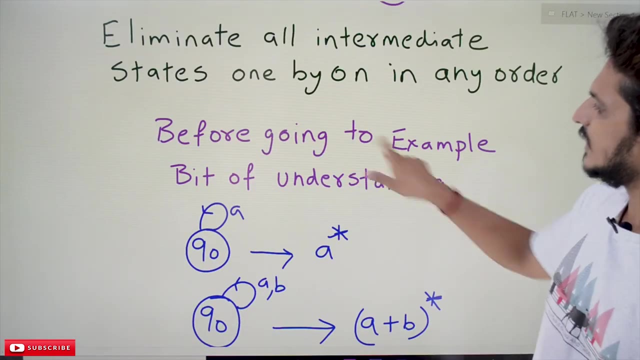 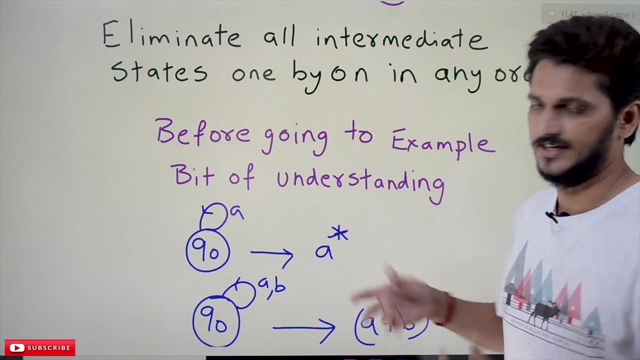 one by one, in any order. We can follow any order in order to eliminate the intermediate states. going to into the example and how to do the elimination process, let's take few general examples. regarding the, regarding the finite automata and equivalent regular expression. with this intuition, you can easily eliminate the states. so for that, to make the process easy, 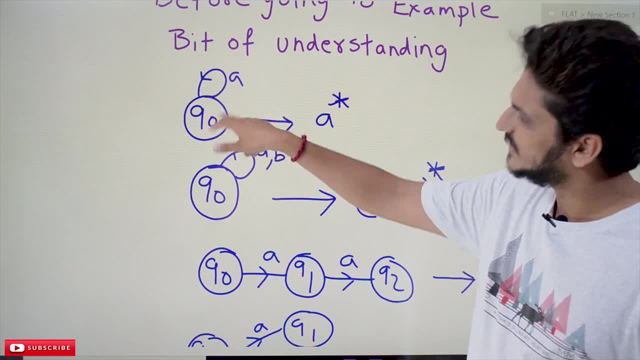 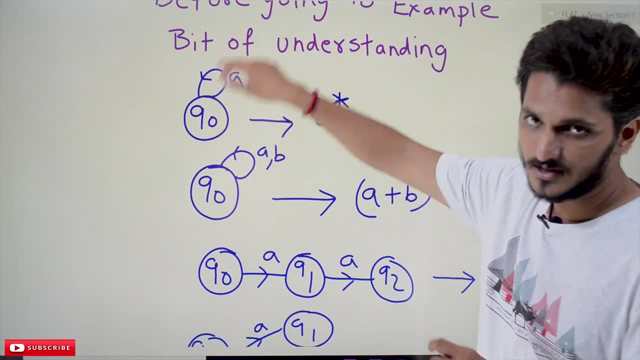 see, if you take an initial state- q naught- and if you assume that this is the final state also, then if you write a thing like this: a if you find a, you are staying on q naught. if you find another a, we stay on q naught. any number of a's this is going to accept, this can be written as a star. 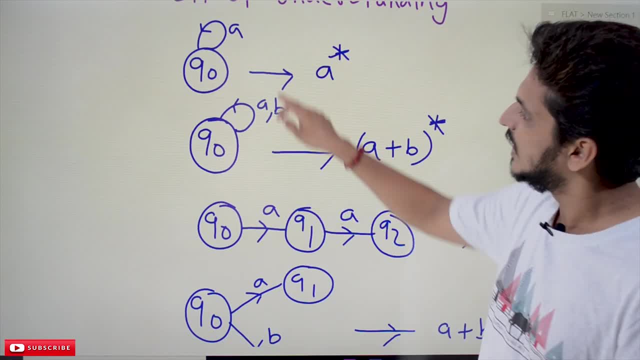 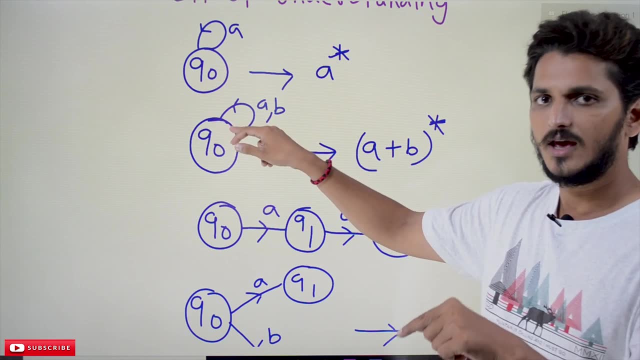 the same way. the next one is q naught. if you take a, we stay on q naught. if you take b, you stay on q naught you can. you can take it in any order: a, b, b, a. so we stay on q naught. this can be written as: 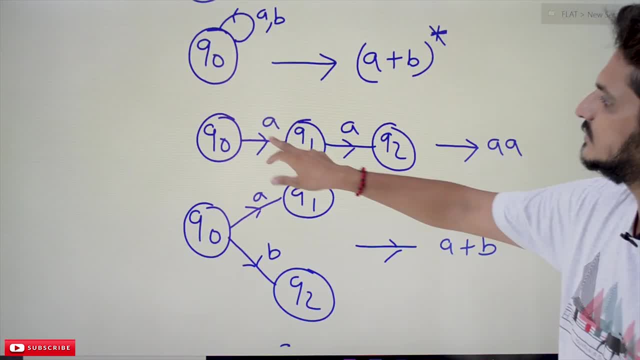 a or b. whole star the same way. next one is q naught. after taking a, we move to q1. after taking a, we move to q2. this can be written as a, a a, similarly r operation. this type of examples we discuss many in our previous classes: q naught. 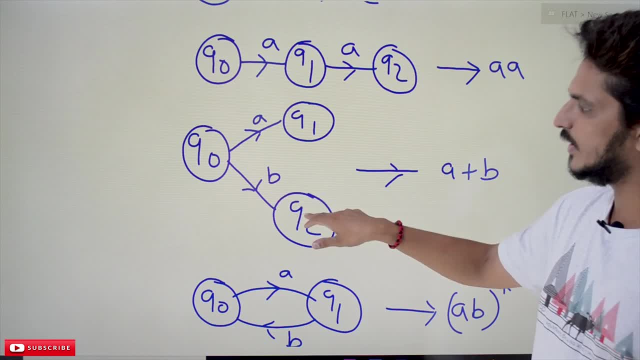 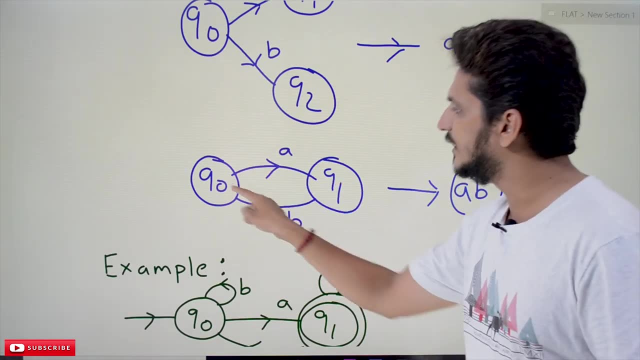 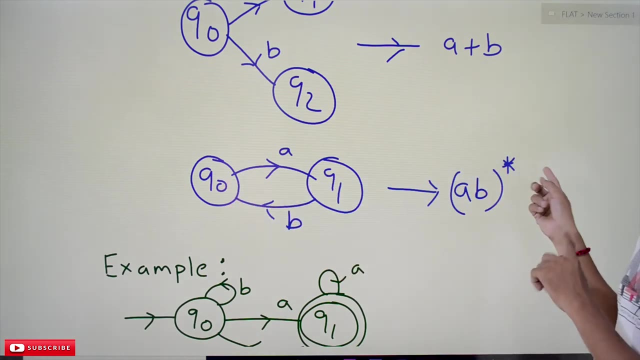 one way we are going to a, one way we are taking b and moving. so this can be written as a or b. that's next one. q naught a, b, a, b, a, b. you can take any number of times. that's why this can be written as a, b, whole star. a, b, whole star. with this intuition, you can easily. 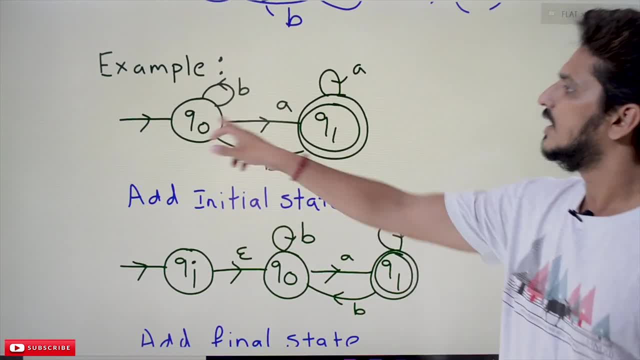 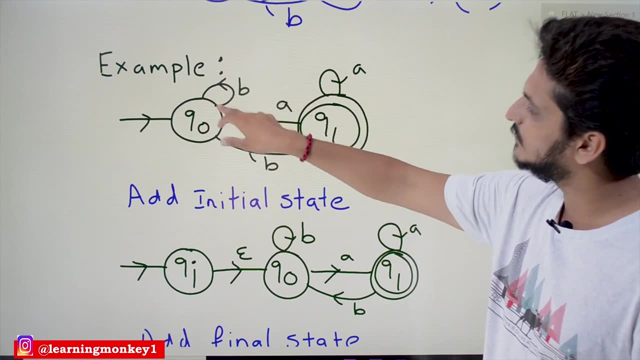 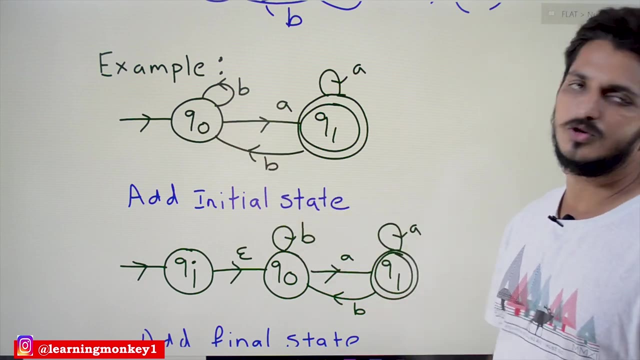 elimination. let's take an example. this is our example. q0 is the initial state, q1 is the final state. so these are the. these are the values we have. on taking b, we stay on q0. on taking a, we move to q1. on taking a, we may move to q1. on taking b, we move to q0. so what's the steps we have to? 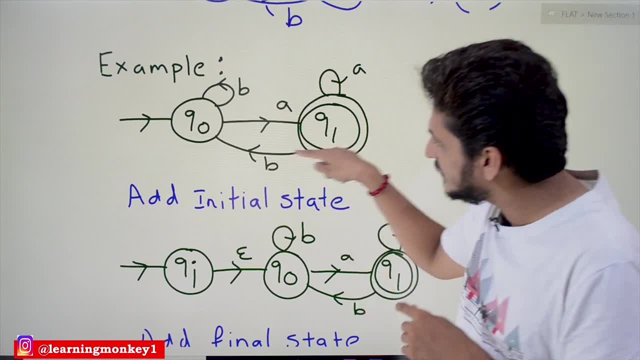 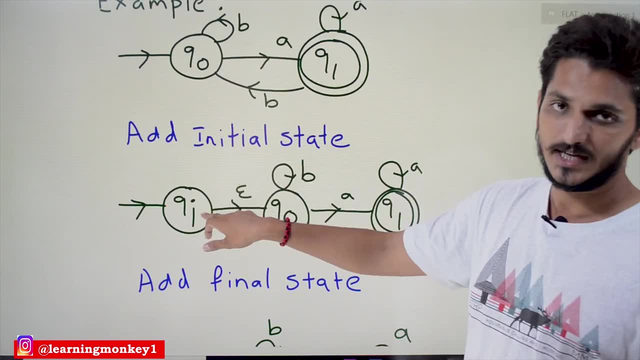 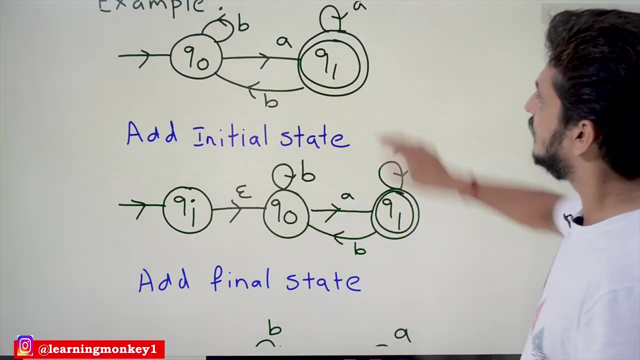 follow. for the first step is: whenever there is an incoming edge to the initial state, add a new initial state. that's why we add a new initial state. we take it as qi. using epsilon moves, we are moving to q0. remaining remaining thing is same. no need to change anything whenever. 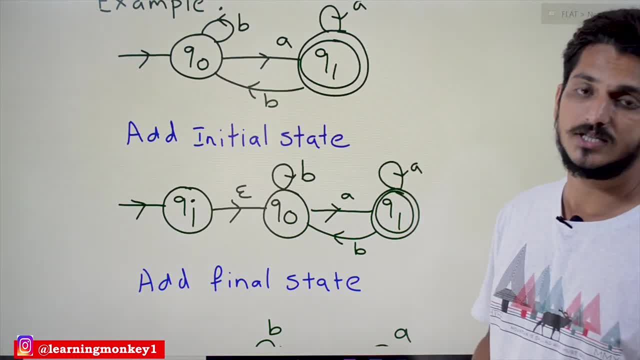 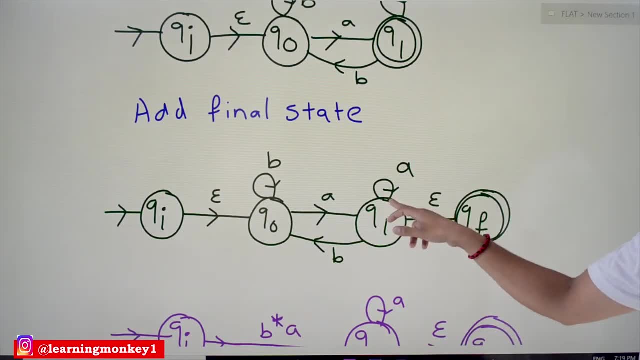 you are having a outgoing edge to the from the final state. add a new final state. add a new final state after adding a new final state. see q1 is the non-final state. using epsilon moves. we are moving to qf. qf is our final state. qi is our initial state. 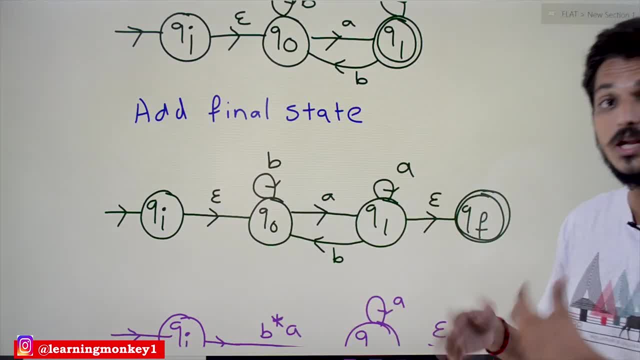 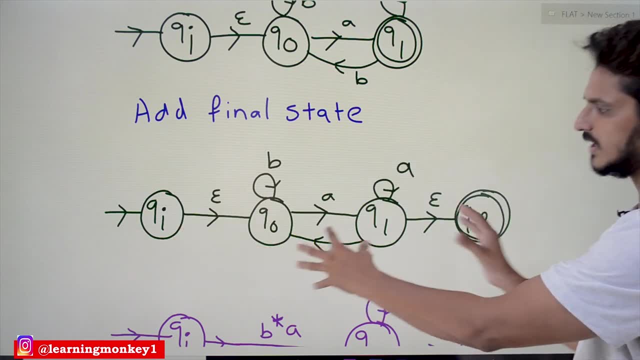 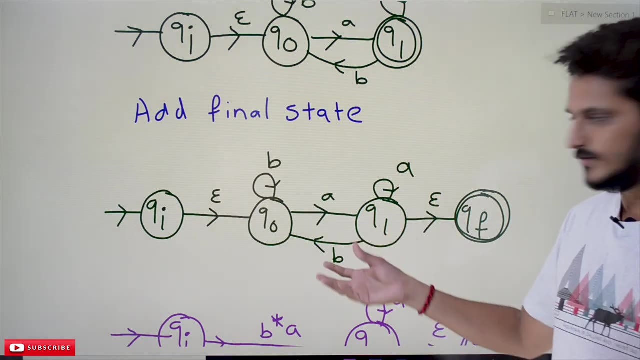 you. Now we are done with the steps. we have to eliminate the intermediate states. what are the intermediate states? q0 and q1, initial state, final state. eliminate the remaining states. that is what you have to do. So here we can do. we can the first one: you can eliminate q0. after that, you can eliminate. 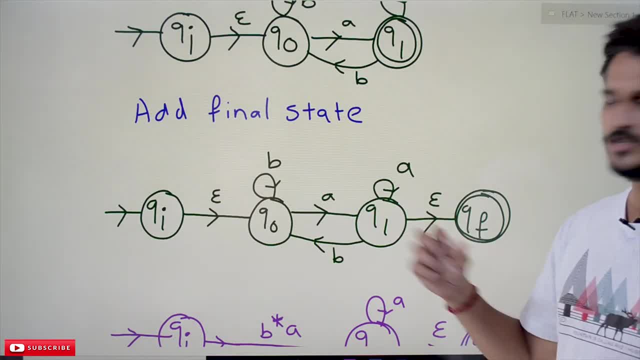 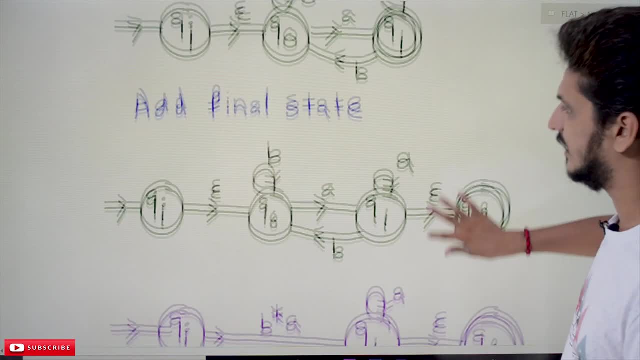 q1. either ways. you can eliminate q1 first, then go with q0. we will show both the ways. any way, you will get the same answer. that is what you have to understand. Let's take this example. this is our final DFA after converting the steps. see if you. 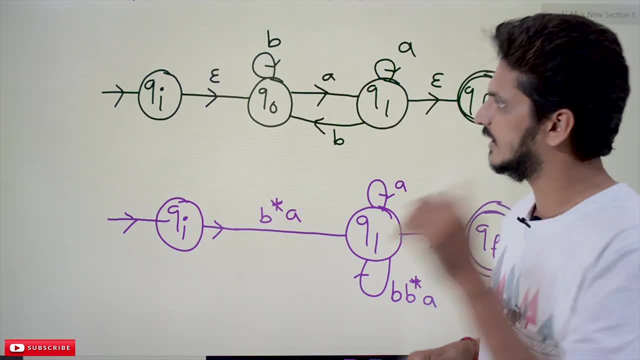 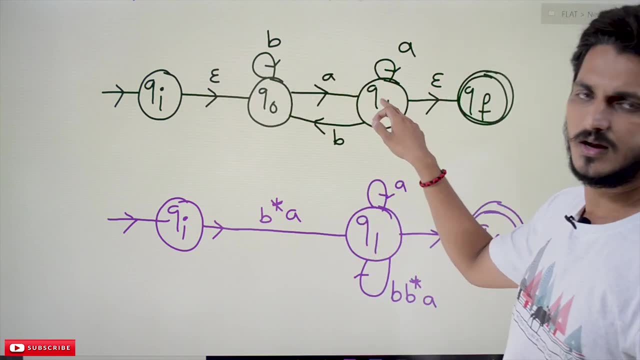 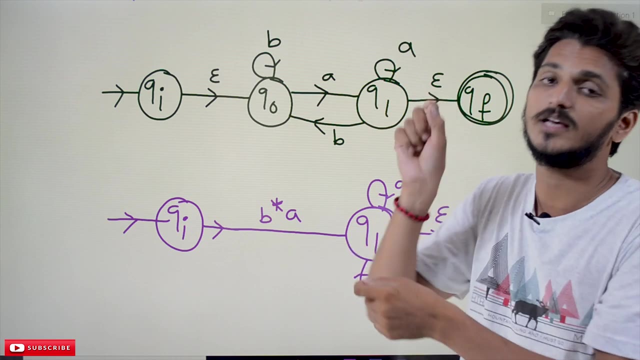 want to eliminate this state, how you have to think this: qi to q1. in between, we are having q0 means from qi. if you want to move to q1 after eliminating this, what's this state is going to do? that is what we have to write it in a regular expression. 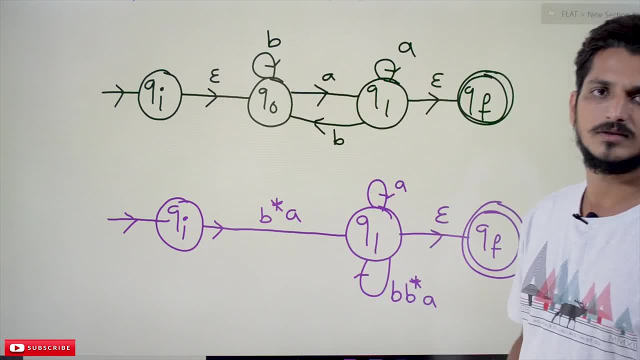 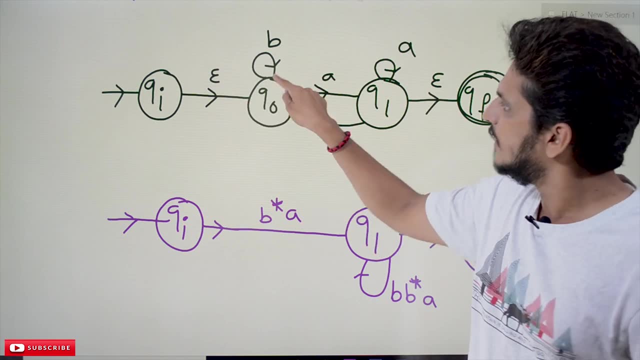 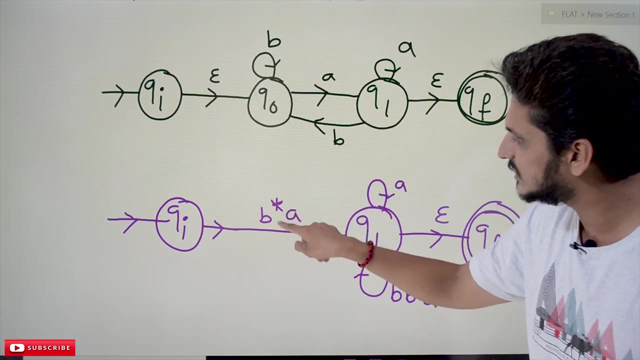 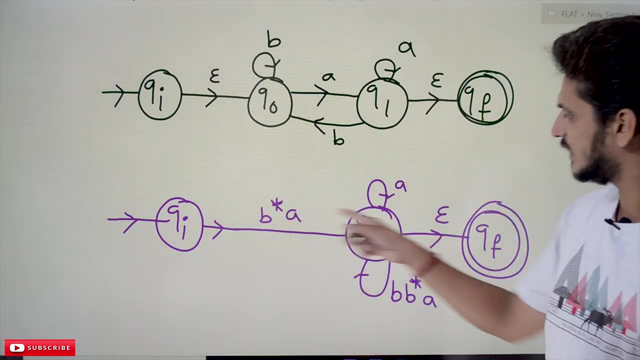 See b star u a. from qi, epsilon we move to here. epsilon means no need to write. that's why we did not mention b star a. we can move from qi to q1.. So that is why b star a, after eliminating q0, b star a, with b star a we can move to q1. 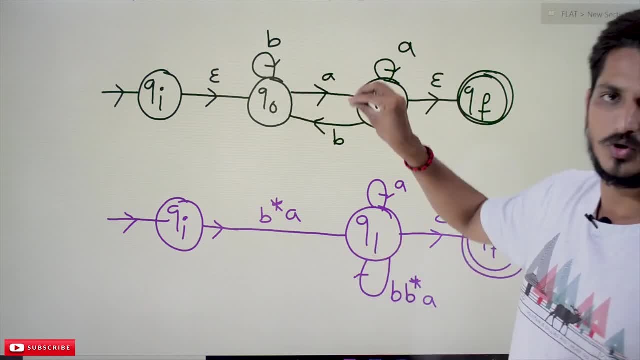 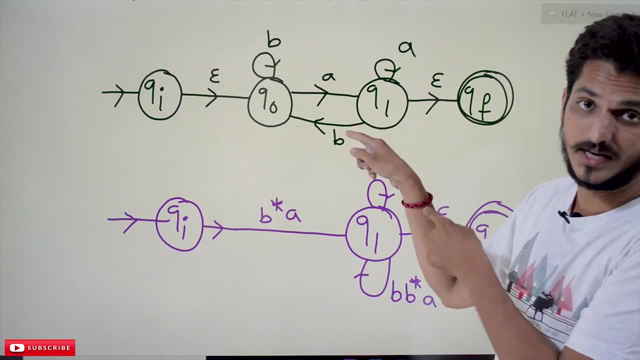 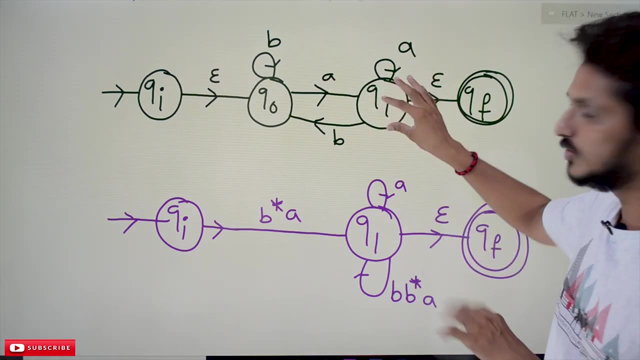 and one more thing you have to remember: whenever you are eliminating q0 from q1, we are having the edge, outgoing edge- to q0, so this should also be taken care of. So b, b, star a, again we are coming to q1. so from q1- again, repeat it- from q1 we are moving. 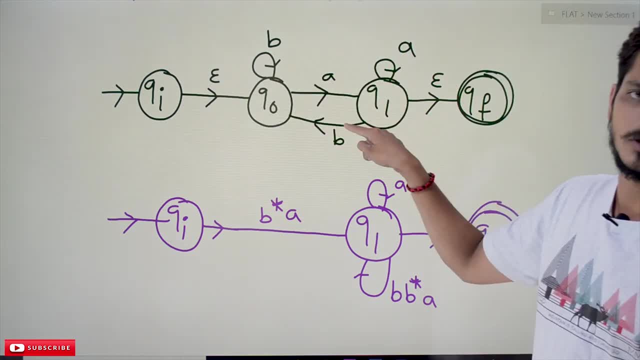 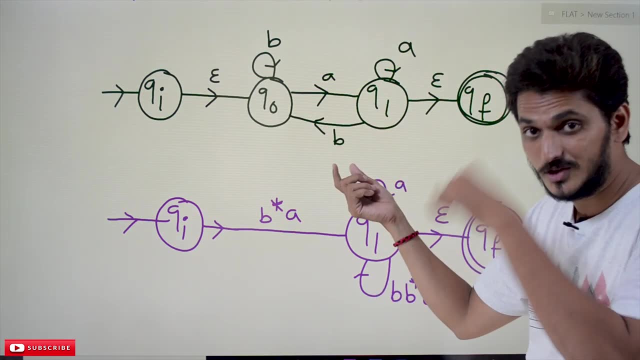 to q0 whenever you eliminate this. you have to take care of this also: what, what, what it should be done. so that's why we have to write the expression for this also. this is the point you have to understand not only one way. you have to check both the ways. 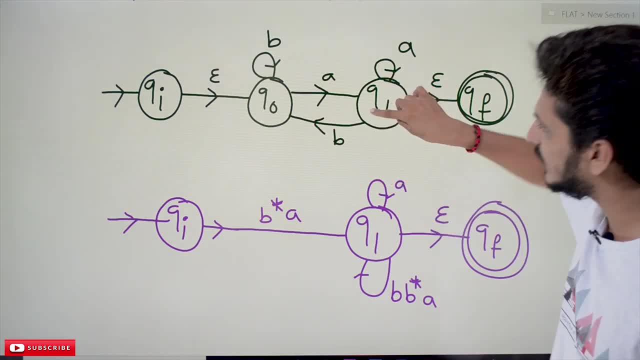 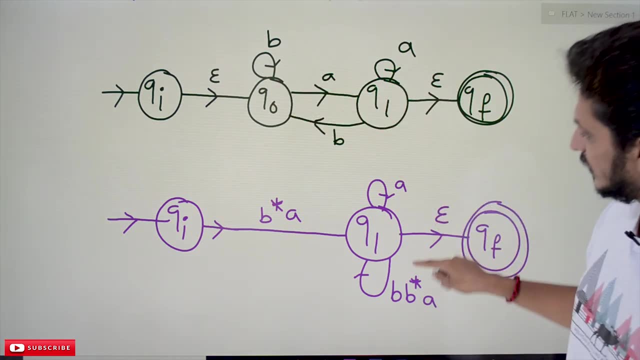 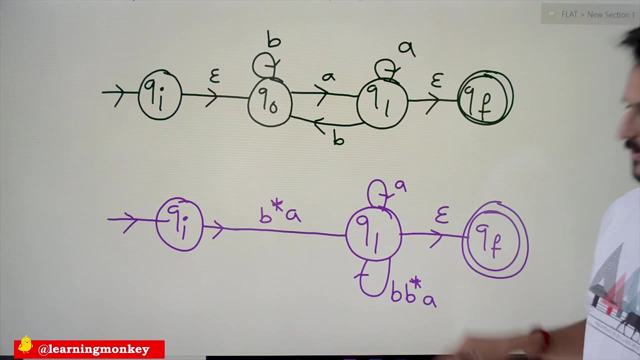 So q1 whenever you take b. so from here q1, you take b b, star a again moving to q1. that's why, after eliminating q0, this is written as self loop. both are same: b b, star a. that is written as self loop. self loop: b b, star a. after eliminating q0, this is the final output. 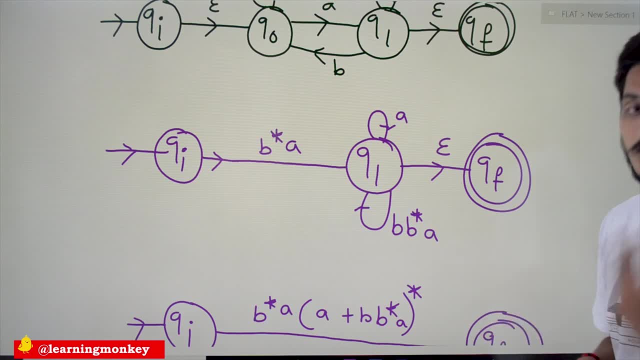 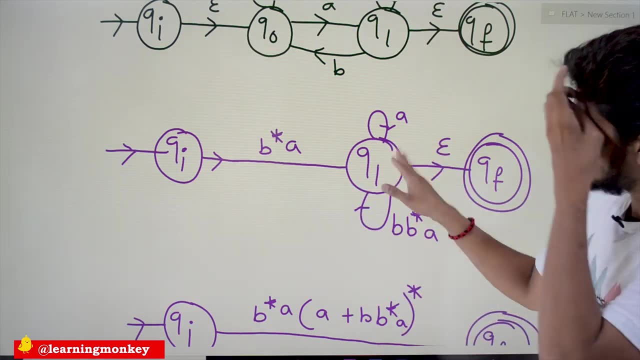 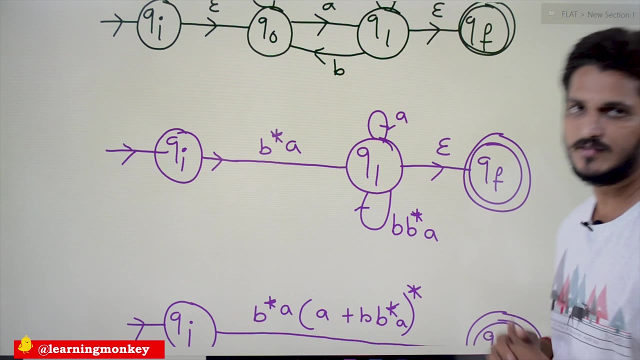 we got after eliminating q0.. Let it understand it properly. then only move to the next step. now we have to eliminate q1, so from qi we can move to q1 using b star a. now, if you want to eliminate this, here we are having two options: a a a, b b star a, b b star a. you can take either a or you can. 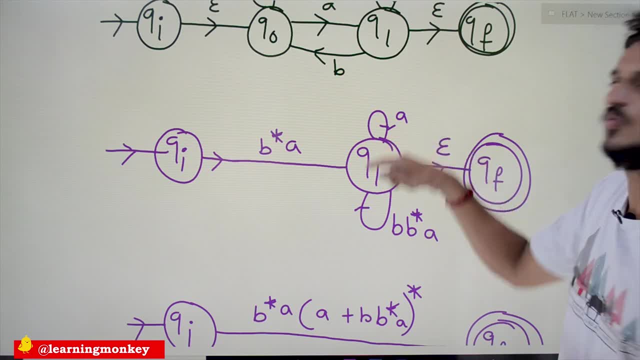 take either b b star, a. anyhow, you are staying on q1. this can be written as A or b b star, a whole or whole. se tone: a, b, b star, the in the above example. we already seen this. similar examples: a or b b star, a whole star. 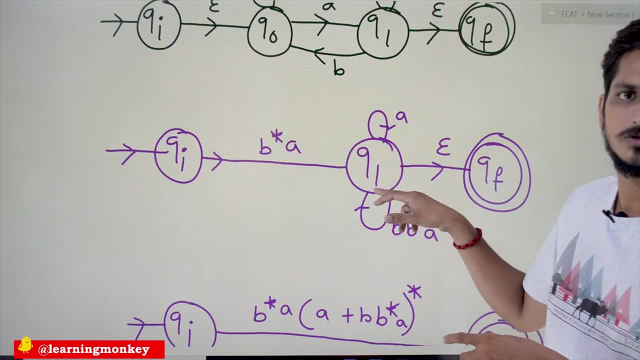 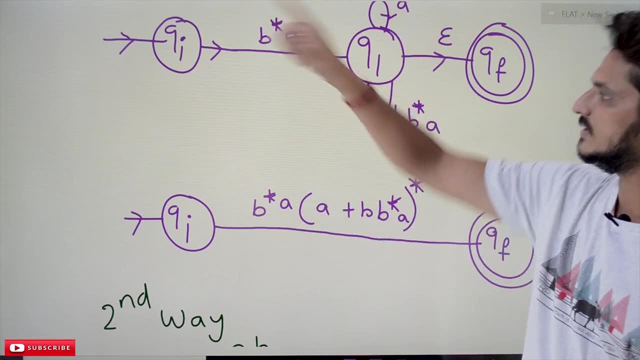 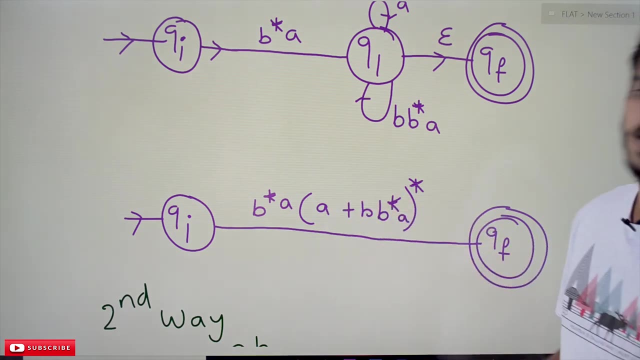 because we are staying on q1. so the final equation we got after eliminating q1 is: so if you eliminate this b star a is obtained previously with that continuation a or b. b star, a whole star. this is the final equation, this is the final regular expression that is going to 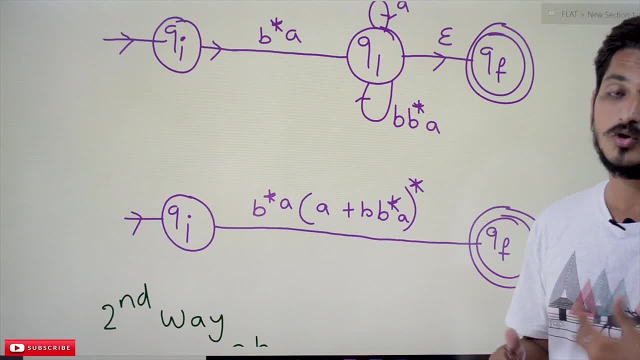 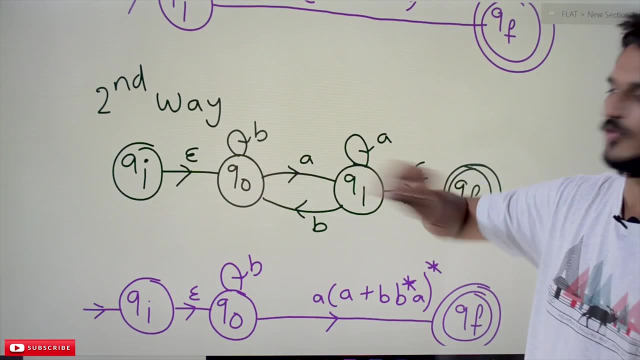 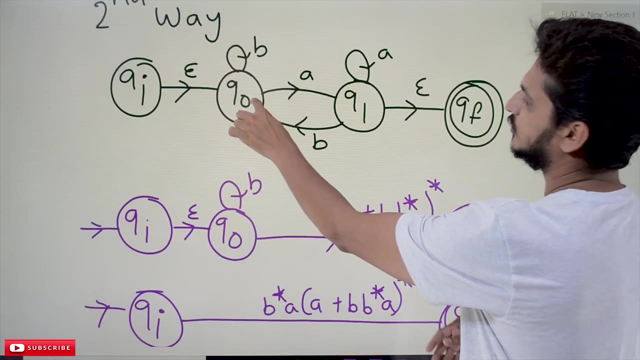 generate for the given df here. this is how you have to eliminate, and we will check the next thing also first. we will second way: we will eliminate q1 first, then we will go with q0 first, q0 second. so this is the example. if you want to eliminate q1 from q0, we have to move to qf. 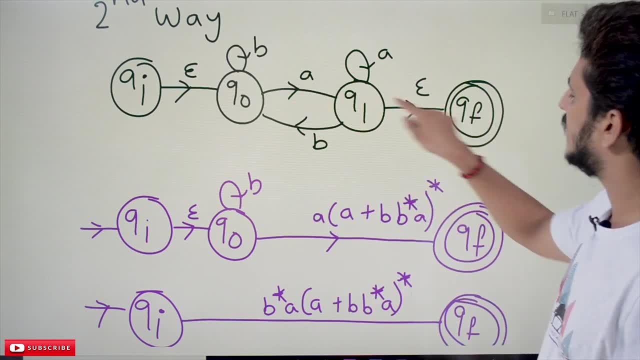 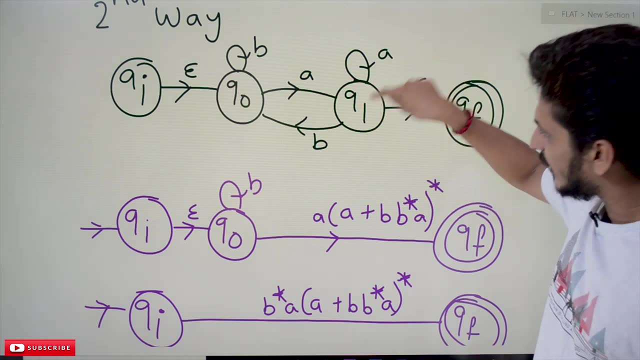 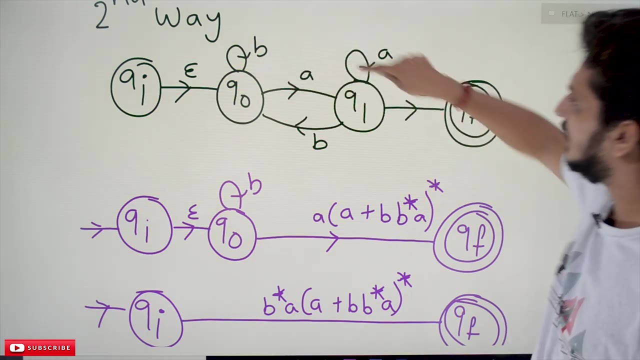 from q0. by taking a, we are we can. by taking a, we are moving to q1. okay, so by taking a, we are moving to q1. q1 from q1. you are having two options: either you can take a any number of times, or b, b star a. 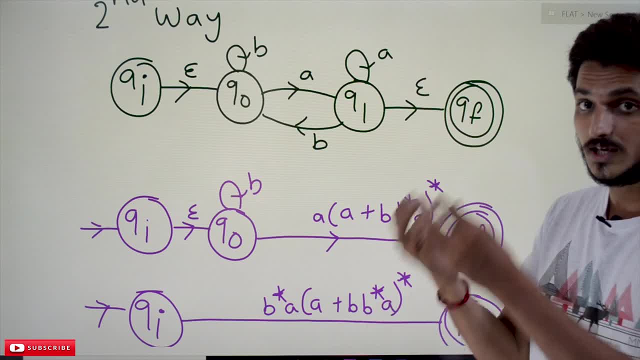 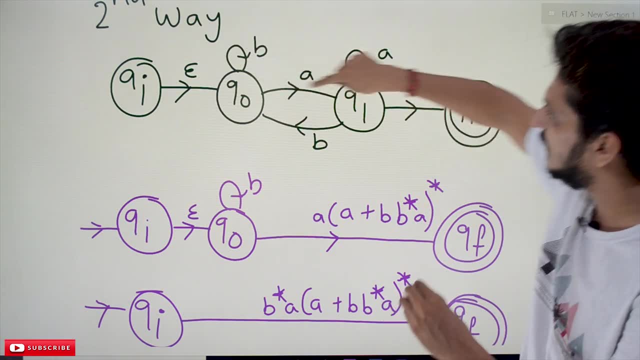 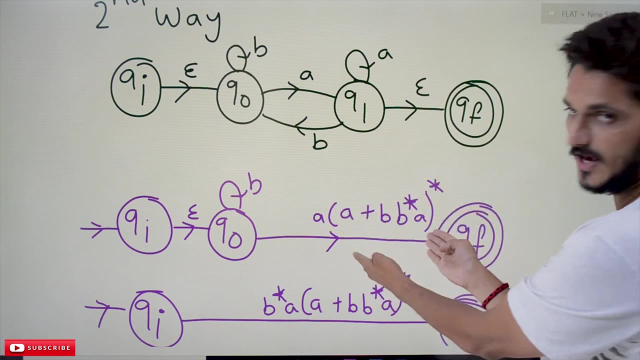 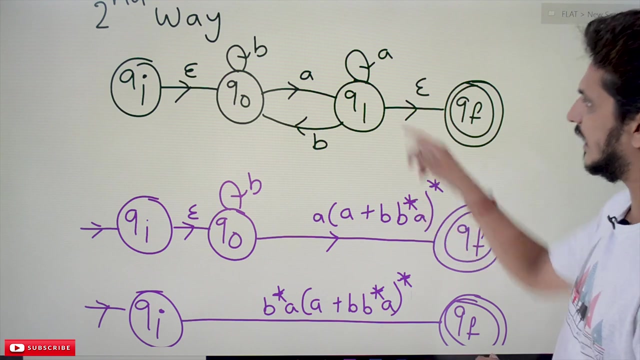 so after taking a you are having two options: a star a or b b star a. again you can come to q1. so this can be written as a. after taking a, a or b b star a whole star. so why a or b b star a? so you stay on q1. you, by taking a, next time you can take b b star a next. 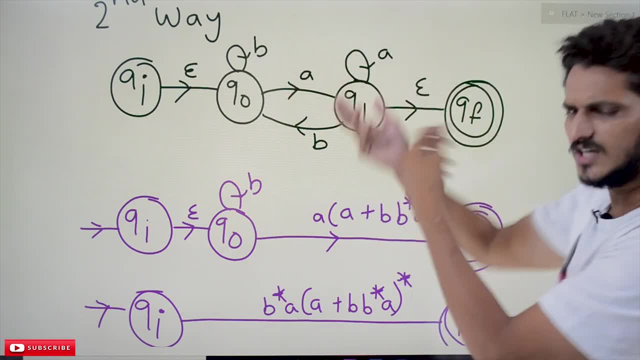 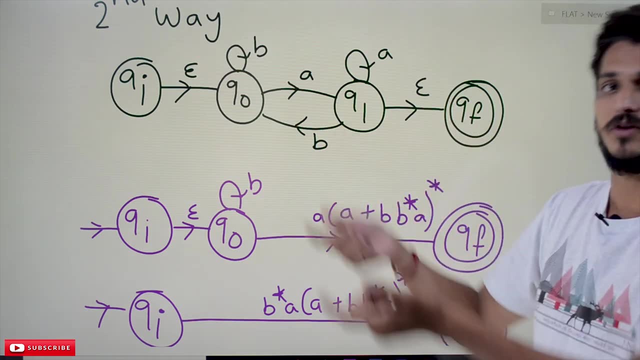 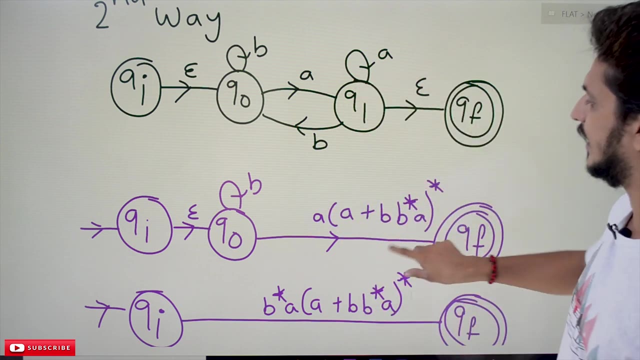 time you can take a. next time you can take b, b star, a like that. any way, you can stay on q1. that's why a or b, b star, a whole star. this can be repeated any number of times. that is why whole star. so this is the expression you got after eliminating q1. so now this is the. this is the. 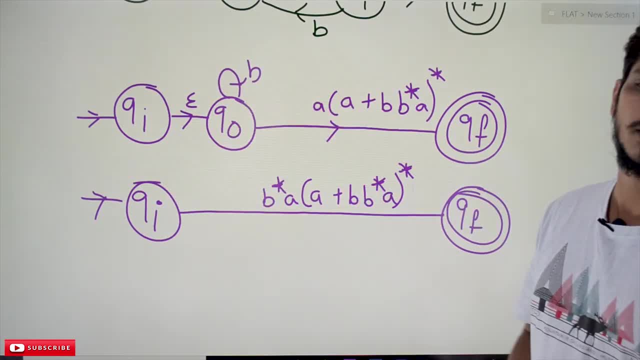 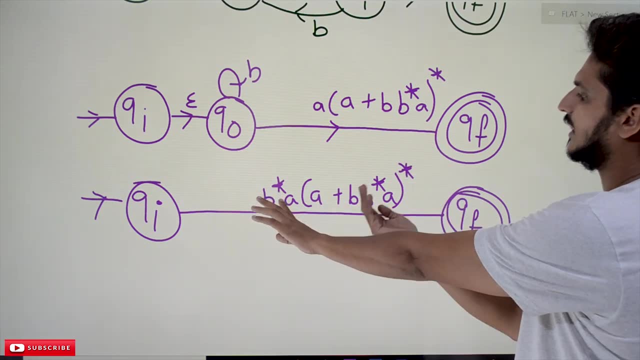 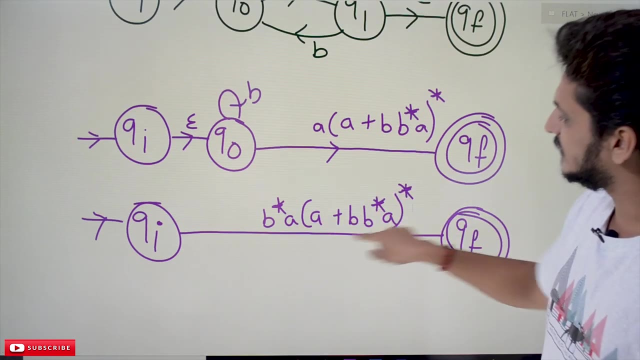 dfa we got. so if you want to eliminate q0, what is this? it's very simple: b star, b star, followed by the previous one is a a plus b, b star, a whole star. the same example we got. the same expression you got. this is the expression we got after eliminating q1 and q0. the same expression we.